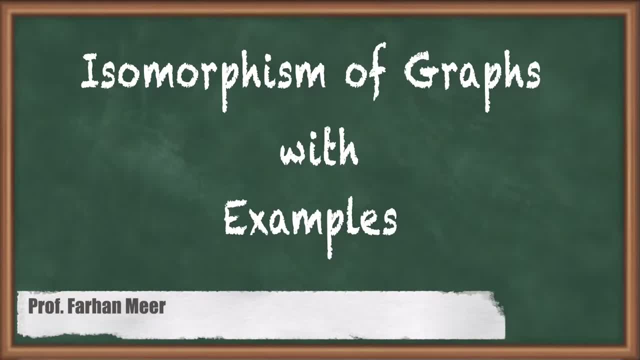 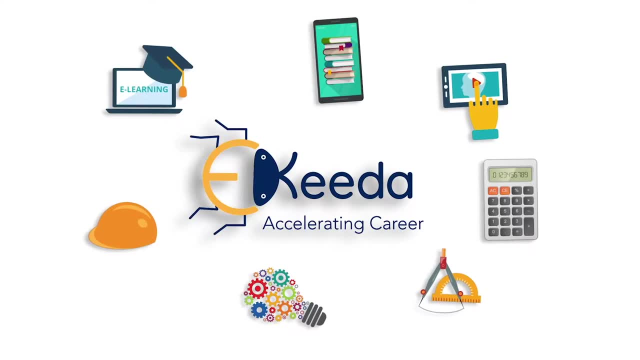 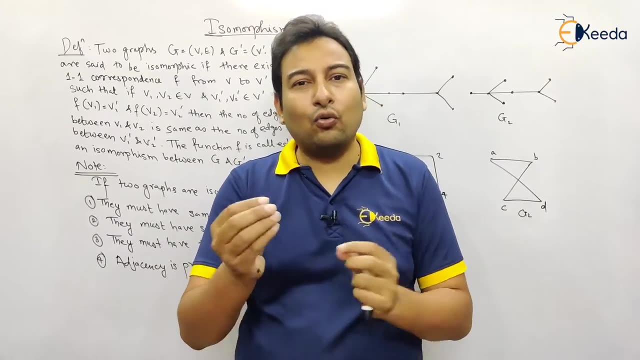 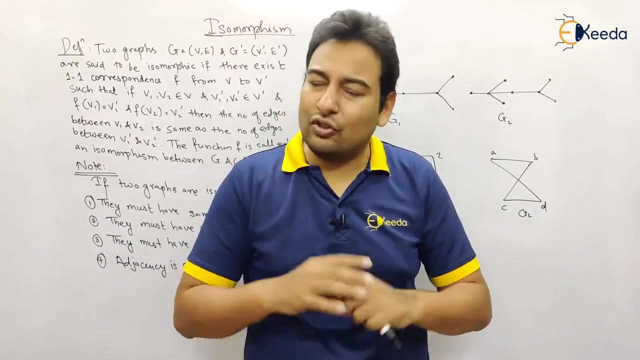 Hello, friends, in this video we'll talk about isomorphism of graph. Welcome back, friends. Let us talk about isomorphism of graphs, a very important topic. Out of 10 papers, you can say 7 to 8 papers, at least 7 to 8 papers. So this topic is very 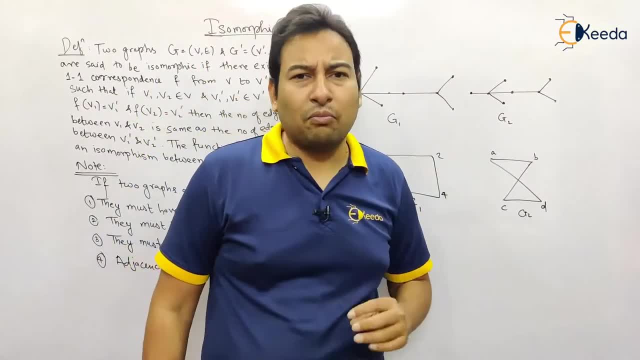 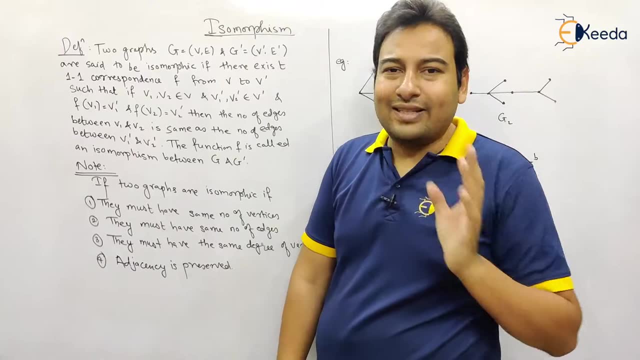 important comes in the exam. So let us discuss- and it's very simple topic. A definition is given here, but it's a very complicated definition. You read it, but I am sure you will not understand anything, So I'll explain you with the help of examples. then it will. 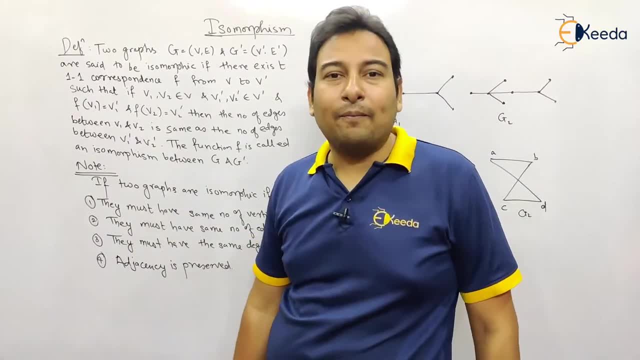 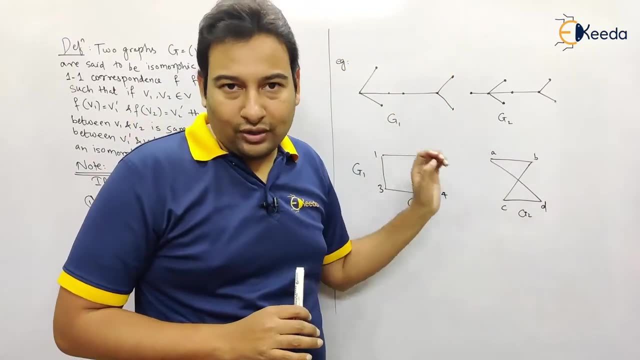 be very clear. So there are four points that need to be satisfied for graphs to be isomorphic. Basically, we are checking whether the two graphs are isomorphic or not. So there are four conditions that needs to be satisfied. The first condition is they must have the 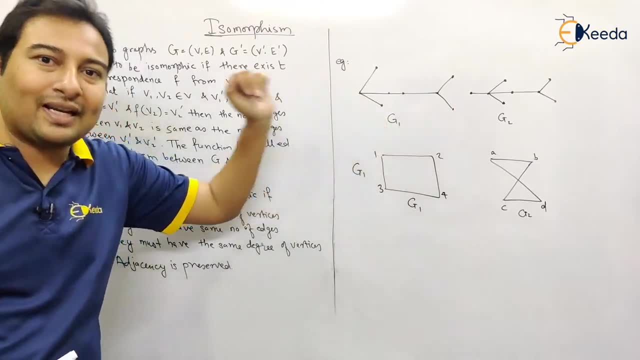 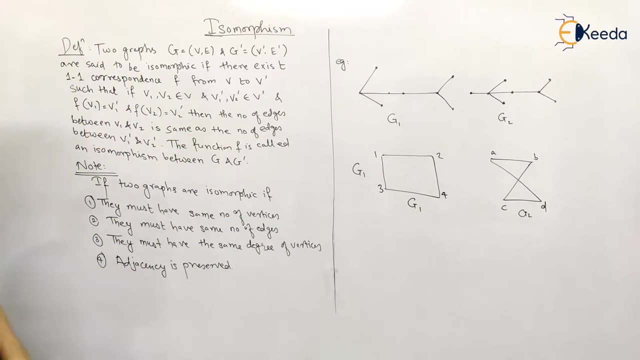 same number of vertices. Both the graph must have the same number of vertices. condition number two: both the graph must have same number of edges. condition number three: they must have the same degree of vertices. and the last point is: adjacency is preserved if these four conditions are. 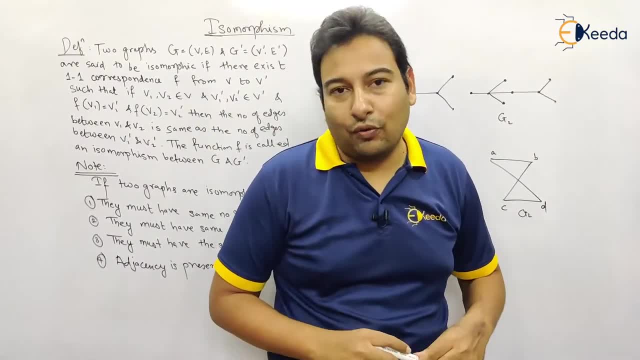 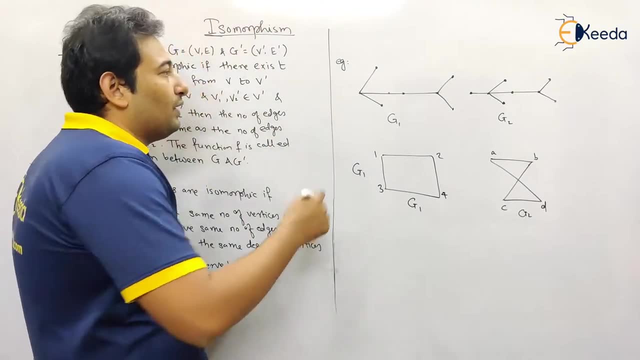 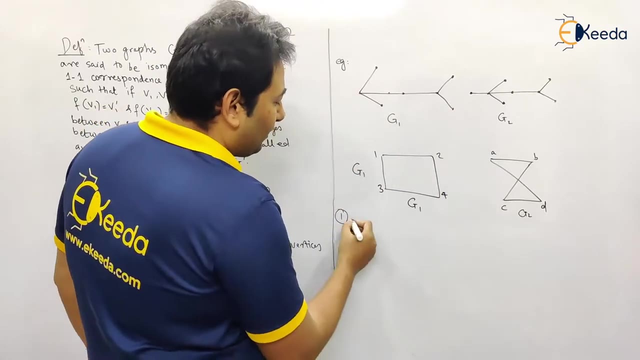 satisfied. you can conclude: the graphs are isomorphic. so let us discuss one by one and let us check these two graphs are isomorphic or not. so let's talk about the first graph. in the first graph, first of all, we need to check number of what number of vertices? so let me check how many. 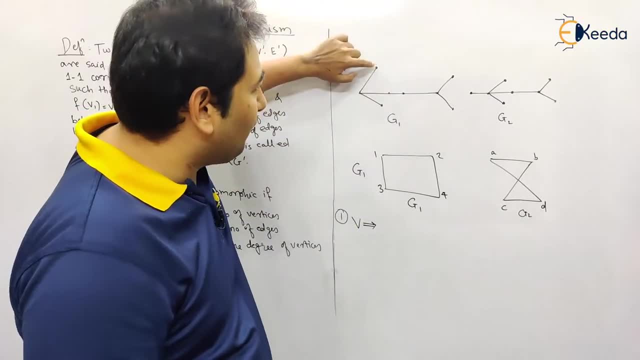 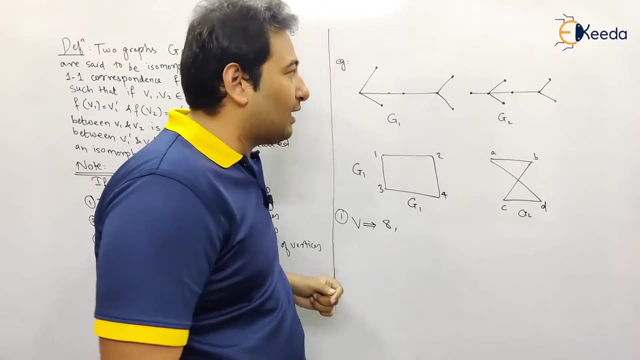 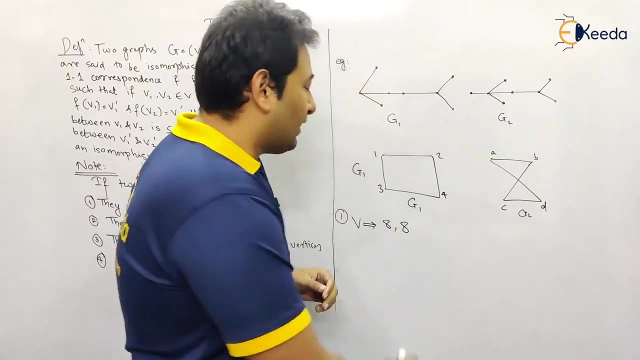 vertices are there in both the graphs. if i talk about the first graph, one, two, three, four, five, six, seven, eight. so there are eight vertices in the first graph. what about graph number two, one, two, three, four, five, six, seven, eight. in the second graph also, there are eight vertices. that means 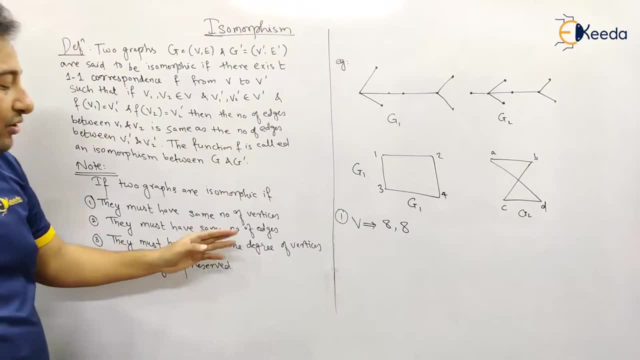 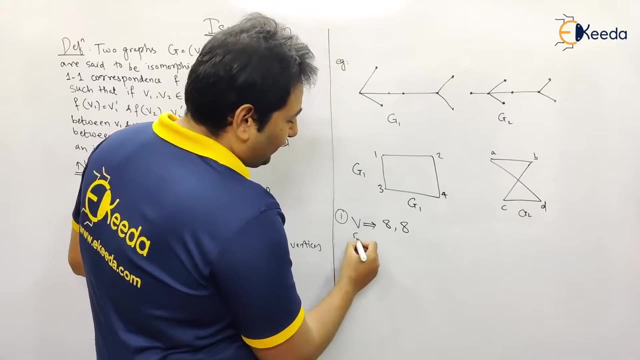 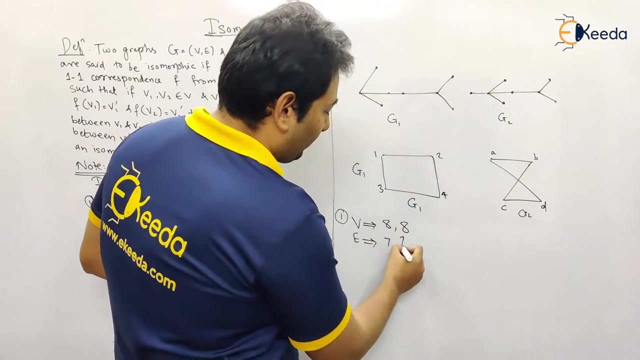 the condition number one is satisfied. the next condition is they must have same number of edges. so here it is: one, two, three, four, five, six and seven. so edges in the first graphs are seven. in the second graph, one, two, three, four, five, six and seven. so number of edges in both. 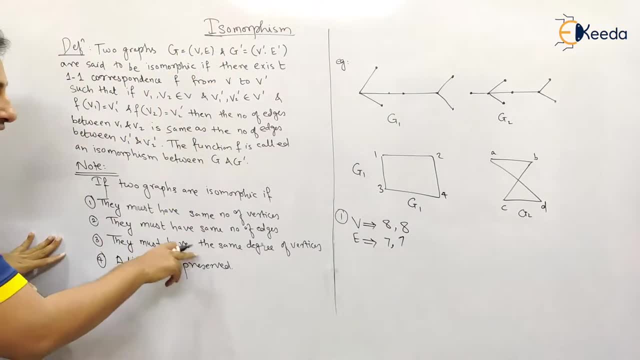 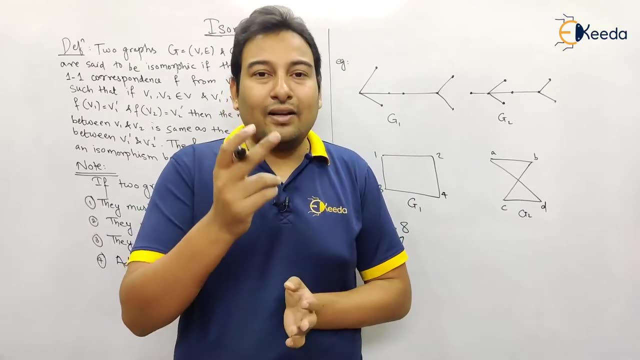 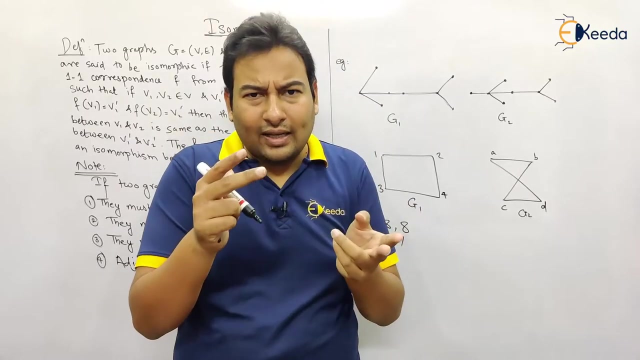 the graphs are also same. condition number two satisfied, they must have the same degree of vertices. they must have same degree of vertices means if in graph number one there are suppose example, giving example, if in graph number one suppose there are two vertices with degree three, any two vertices with degree three in graph number 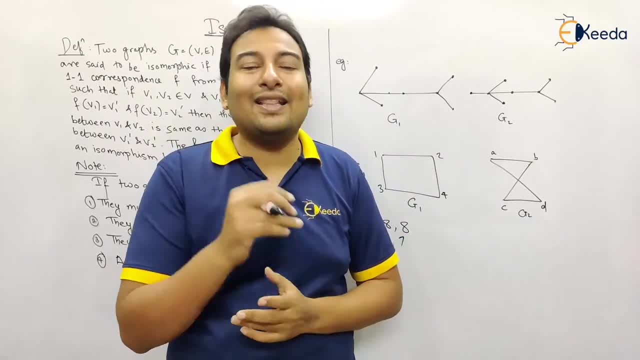 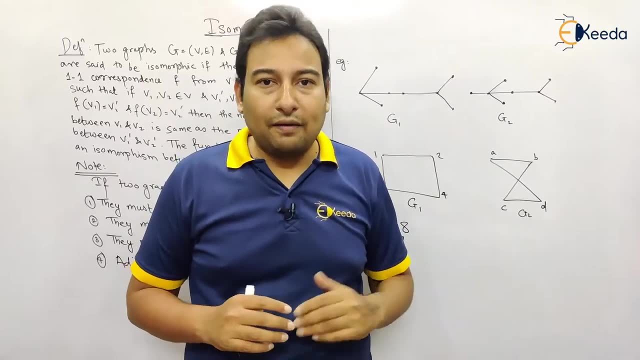 two: also there should be two vertices with degree three. suppose in the first graph there are four vertices with degree five, in the second graph also there should be four vertices with the degree five. so this is the you can say point number three. so let me check if we talk about. 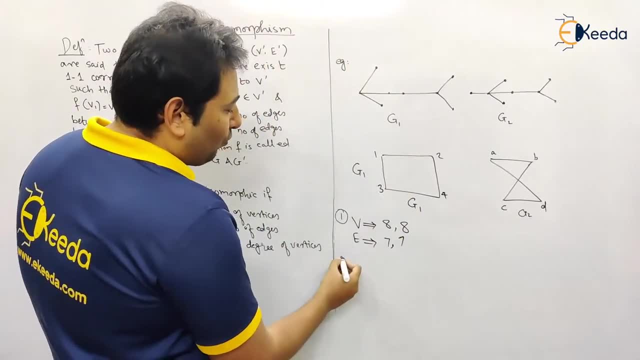 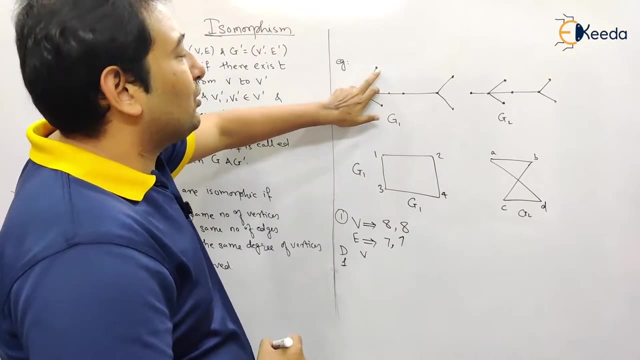 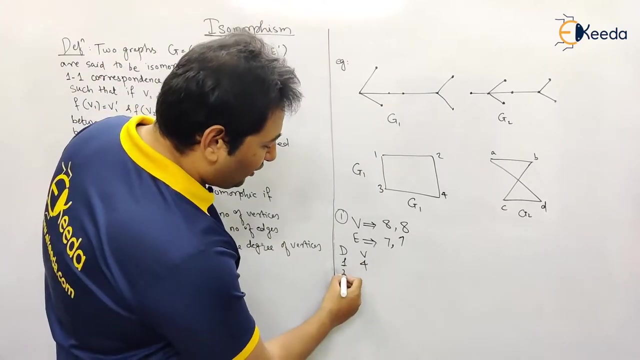 graph number one. in graph number one, let me check how many vertices with the degree one, with the degree one, how many vertices we have. let me check. so this is your text with degree one. this is one. this is one. this is one. that means there are four vertices with degree one. let me check how. 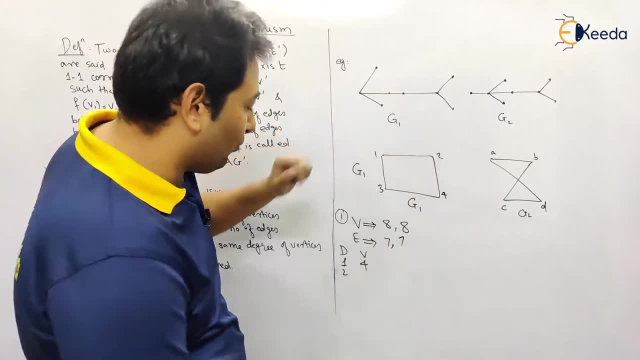 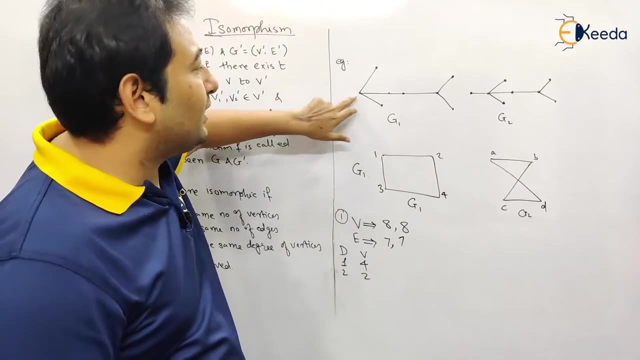 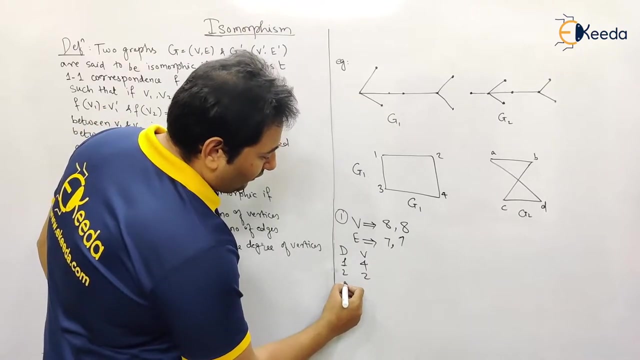 many vertices with degree two. this is your degree two, this is your degree two. so two vertices with degree two, next three vertices. three vertices with degree three. so this is your degree three and this is your degree three. that means degree three. two vertices, same pattern i should get in g2. that means in graph number two also. 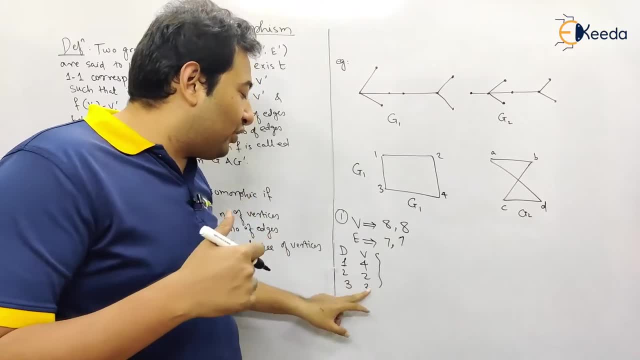 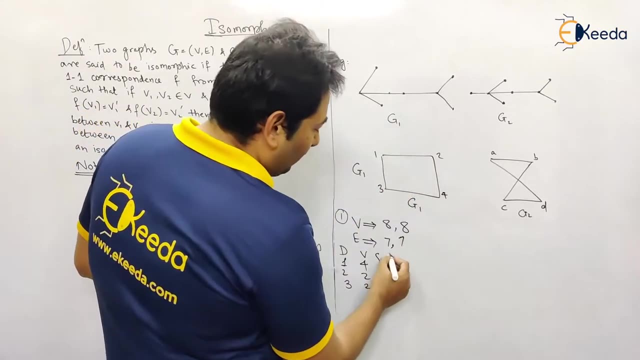 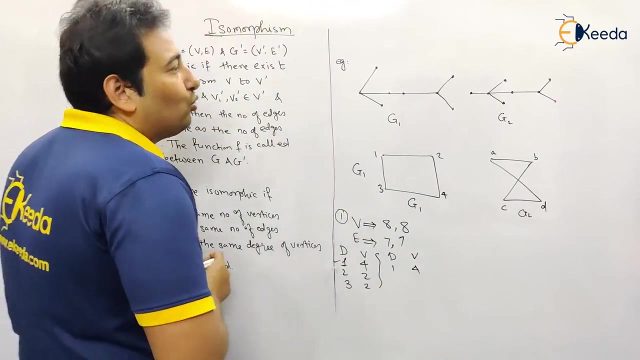 there should be four vertices with degree one, two vertices with degree two and two vertices with degree three. if i'm going to get it, i will say point number three is satisfied. let's talk about graph number two. one degree one, two, three, four, see here. it's same. next, two degree. 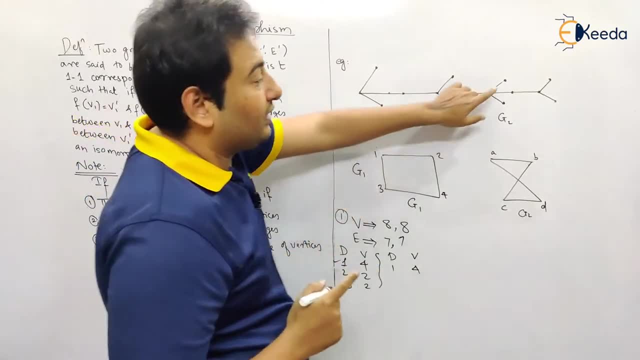 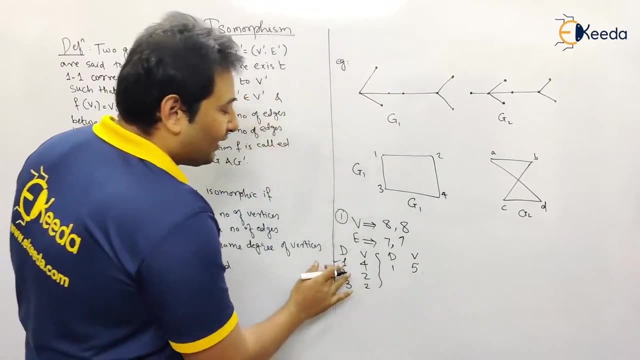 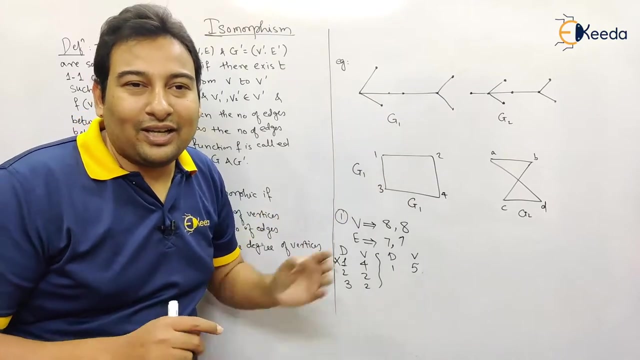 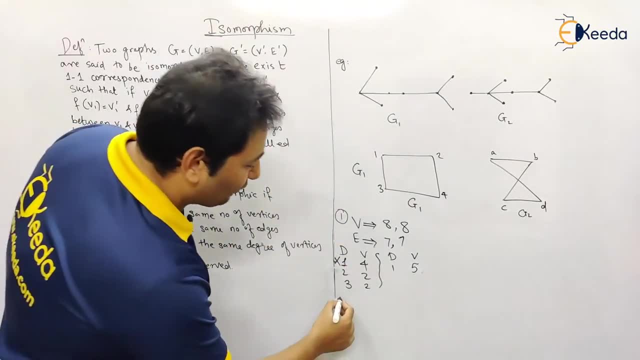 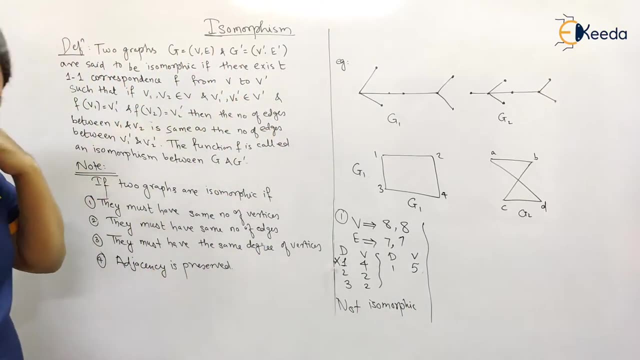 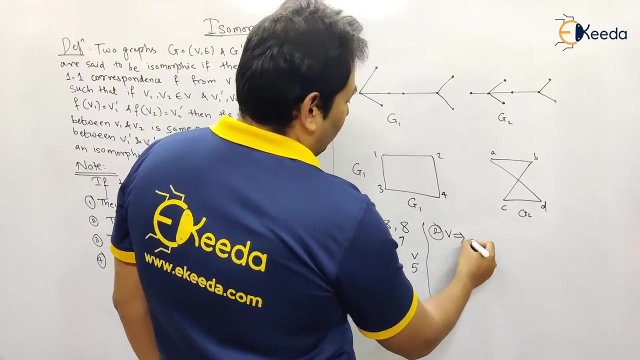 means. condition number three is not satisfied. story over. not isomorphic, is this clear? so this is your not isomorphic graph let's talk about, let's check, uh, the second graph. let me check. number of vertices: obviously four. it's very simple. if you check here, there are: 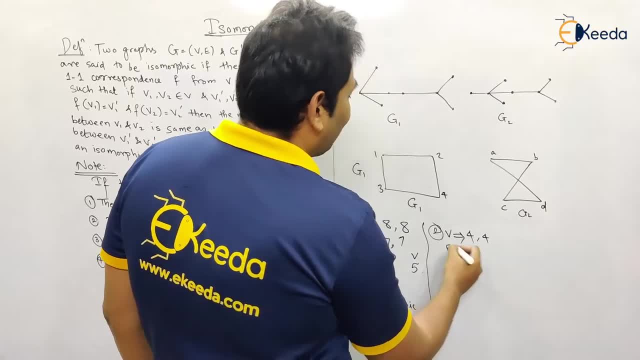 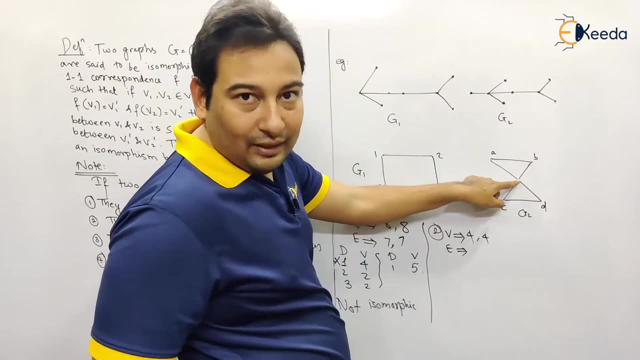 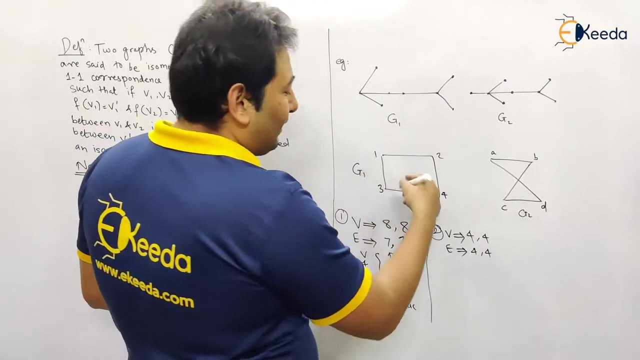 also four. number of ages: how many ages are there? one, two, three, four? if you talk about one, two, three and four, this is your one age. there is no connection here. so one, h, one is in short four ages. both. number two condition also satisfied. if we check, all the vertices are of degree two, see: 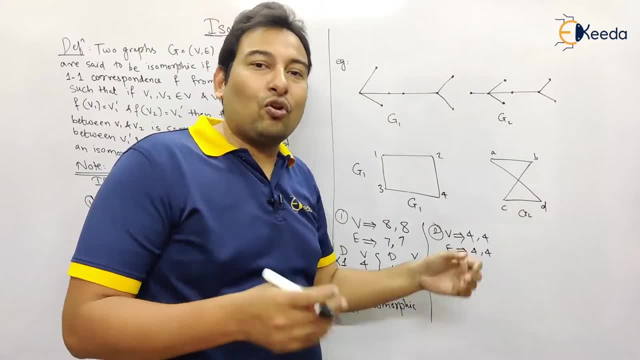 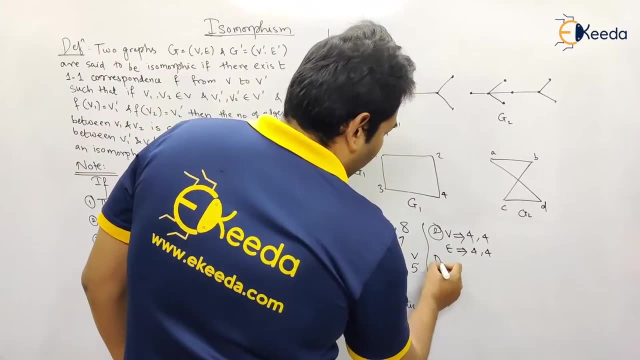 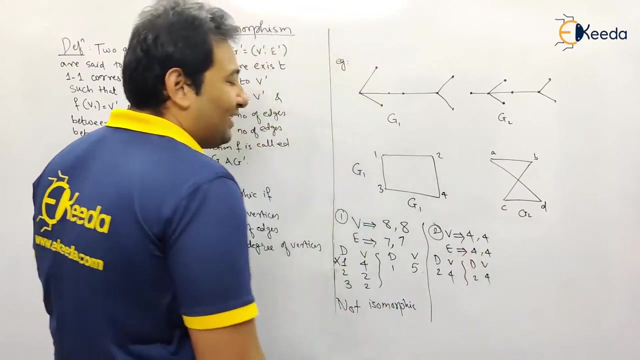 here, and if we check this diagram also, here also all the vertices are of degree two. that means, condition number three is also satisfied, see degree two. how many vertices four? here also degree two. how many vertices four? condition number three is also satisfied. now let us check about condition number four. adjacency is preserved. 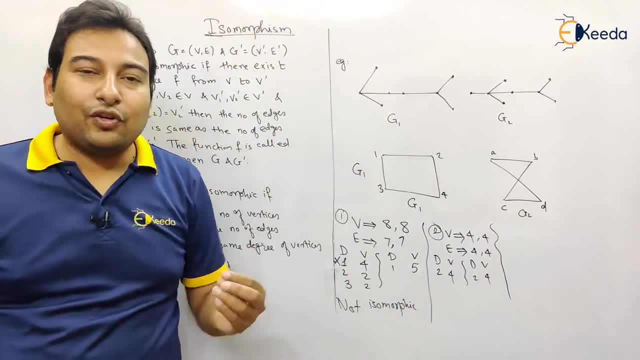 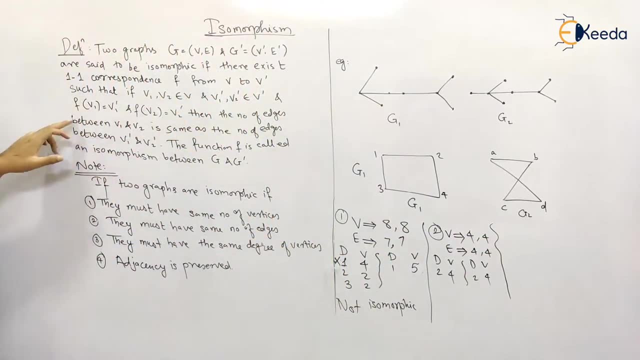 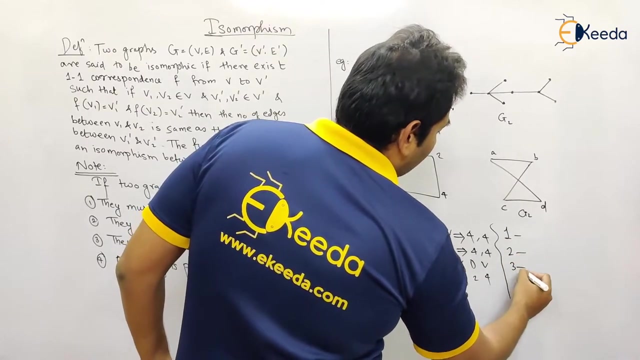 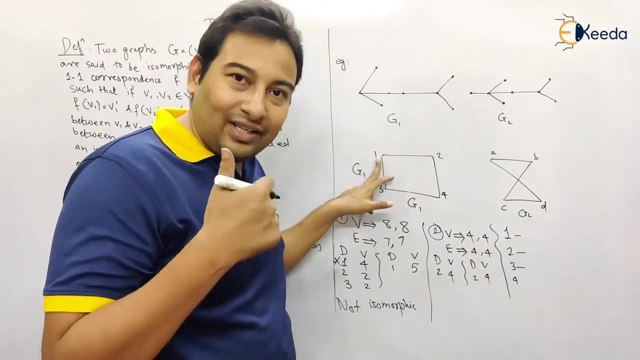 adjacency is preserved means we should be, we should be able to show one-to-one correspondence between the two graphs. one-to-one correspondence means one-to-one correspondence means we should be able to rename it. we should be able to rename it. one, we can rename it as see. one has degree to. let me check. 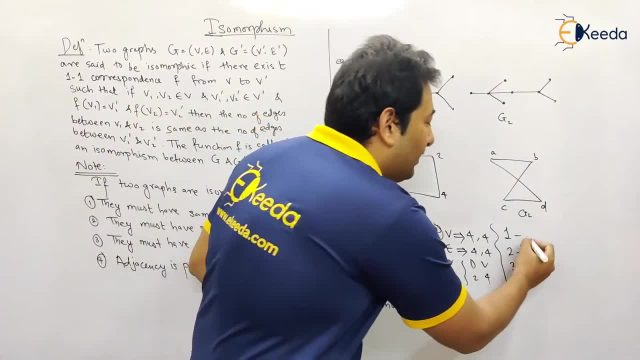 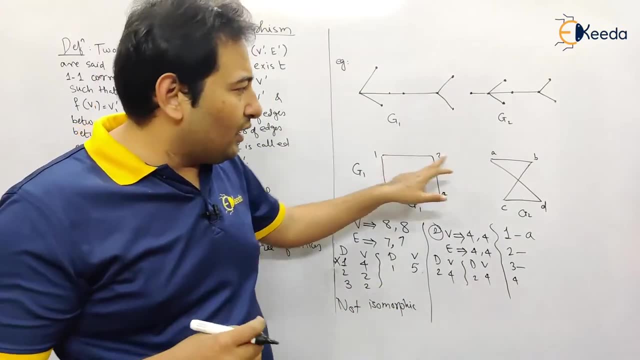 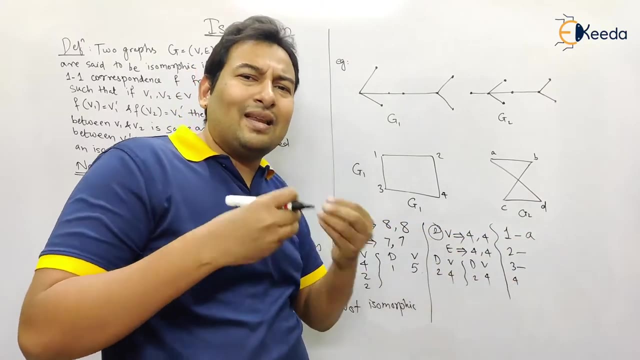 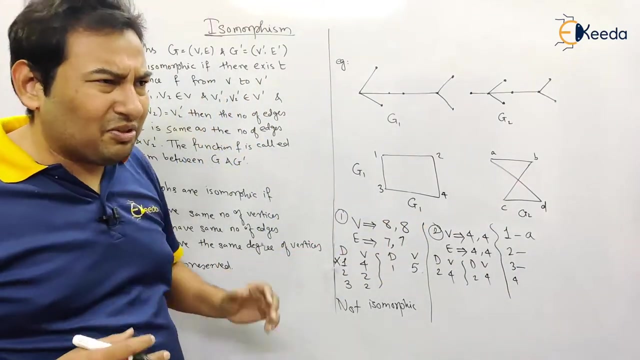 which has degree to a, so one can be rename it as a. now you saying you might be thinking here it is one degrees to. all other are degree to. so can we have b for this? yes, you can have b for this. you can rename any term so one can be a, b, c, d, because both the degrees are same. also, adjacency is. 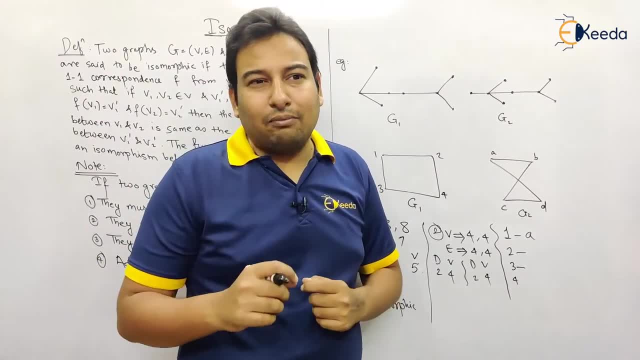 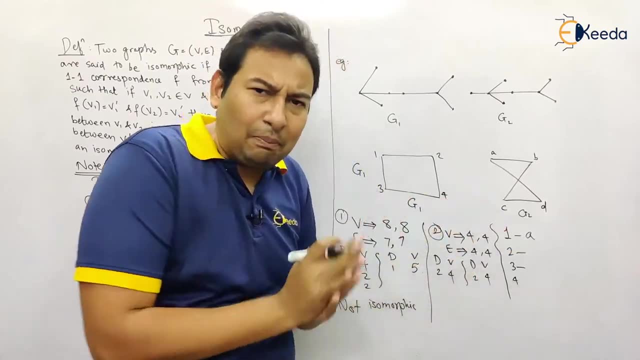 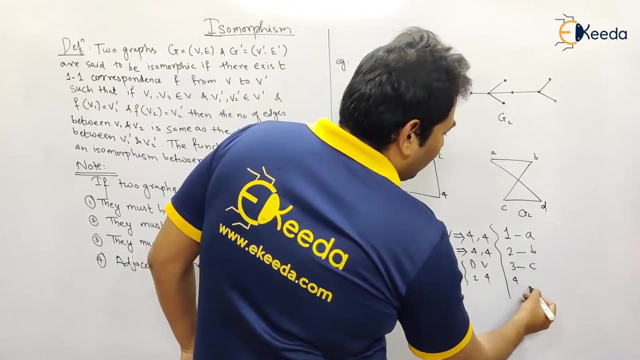 preserved adjacency is a concept that will require a bit more. you can say verification. so about that we're going to discuss in the next video in detail. this is very simple problem. therefore we are not focusing on it. so two, 2 can be renamed it as b. 3 can be renamed it as c and d can be renamed it as d. 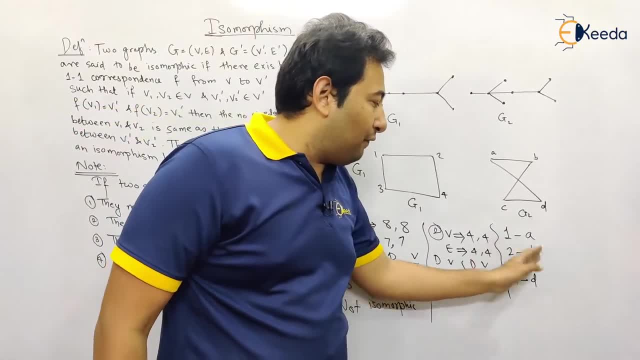 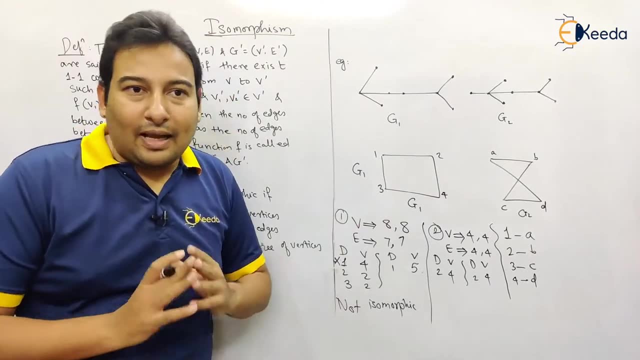 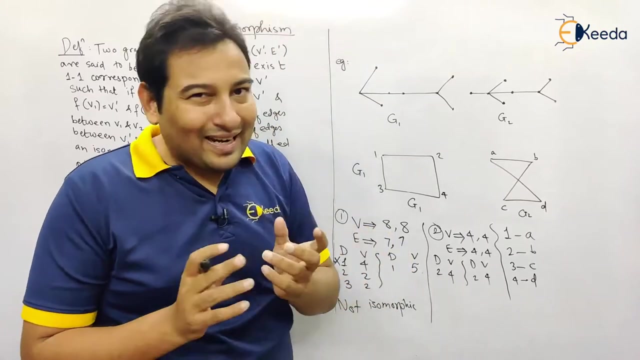 if we can do this, then we'll say the graph is isomorphic. see from this particular example. i'm sure you understood three points completely. what are the three points? number of ages, number of vertices and same degree of vertices. fourth point: adjacency is preserved. there are few more things.